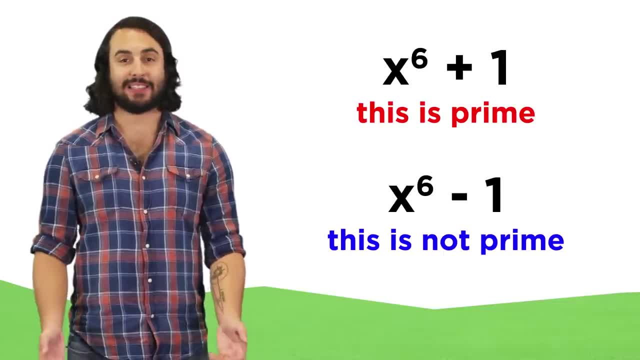 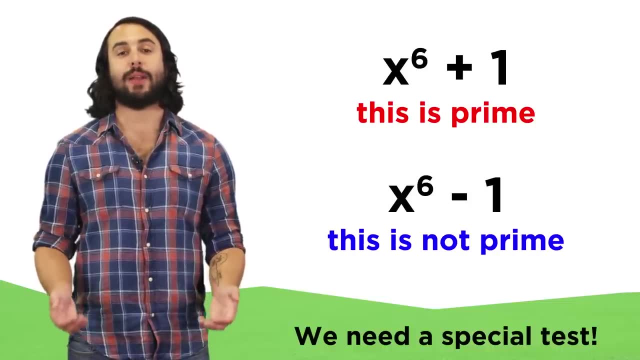 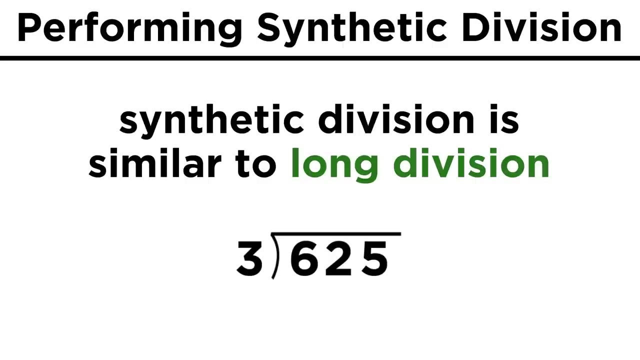 But X to the sixth minus one is not prime. it can indeed be factored. So we need a way to test whether a polynomial is divisible by a particular expression or not. That technique is called synthetic division. It works a lot like long division, which we learned at the beginning of this course, except 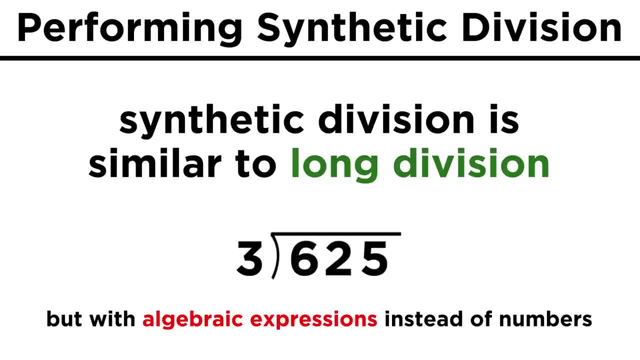 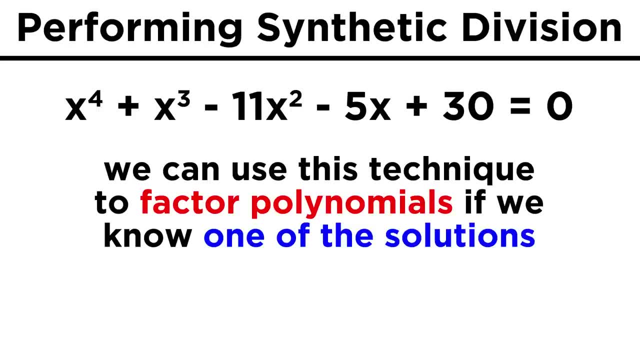 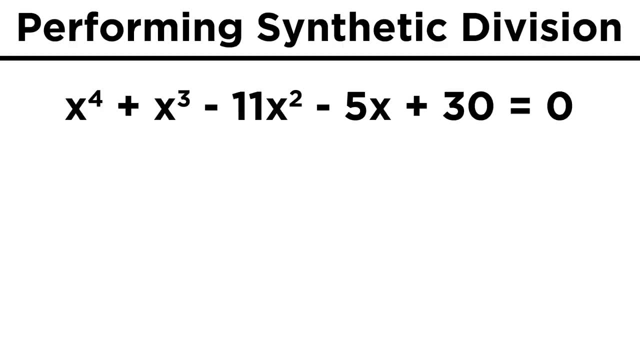 that we are using algebraic expressions instead of numbers. This will come in handy if we have something like a cubic or quadrangle. Let's say we are looking at X to the fourth plus X, cubed minus eleven, X squared minus five, X plus thirty, and we want to see if X equals two is one of the solutions. 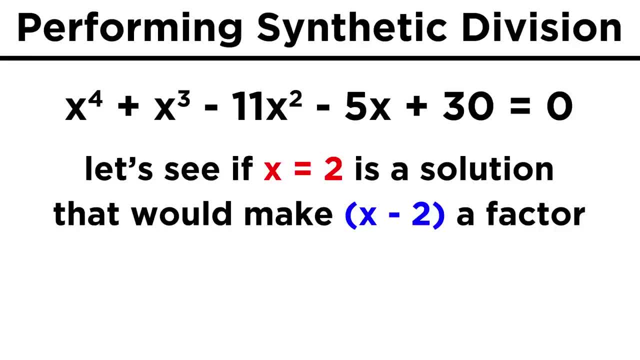 If it is, then X minus two would be a factor, and that could allow us to simplify the expression. The way we will test this is as follows. Let's make two lines at a right angle like this: Let's make two lines at a right angle like this: 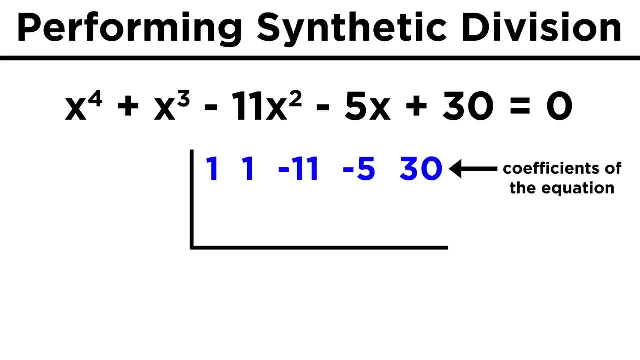 In the top row we will list only the coefficients of our equation. Then we want to test to see if two is one of the solutions. so let's put a two to the left over here. Now we take the first coefficient, in this case a one, and drop it down here. 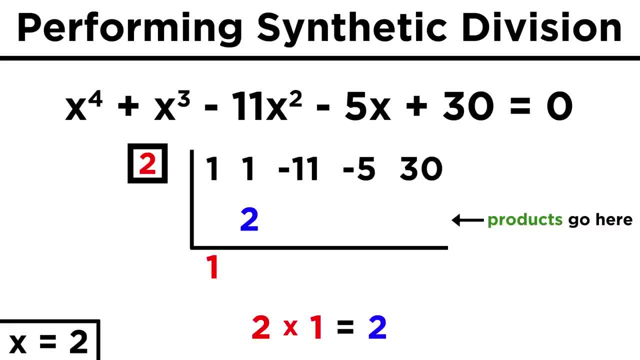 Now we multiply by the two and put that here. Now we can add these together to get three and write that here Again. we multiply by two to get six. Adding to negative eleven. we get negative five. Then we multiply to get negative ten, add to get negative fifteen. multiply to get negative. 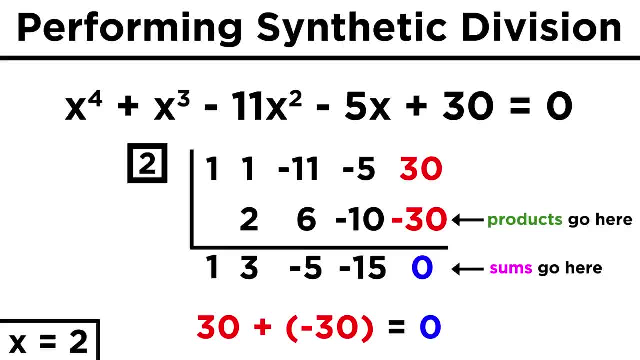 thirty and finally we add to get zero. The fact that this is a zero right here means that there is no remainder from the division, which means that two is a solution, and therefore X minus two is indeed a factor of this polynomial. These resulting numbers here tell us the coefficients. 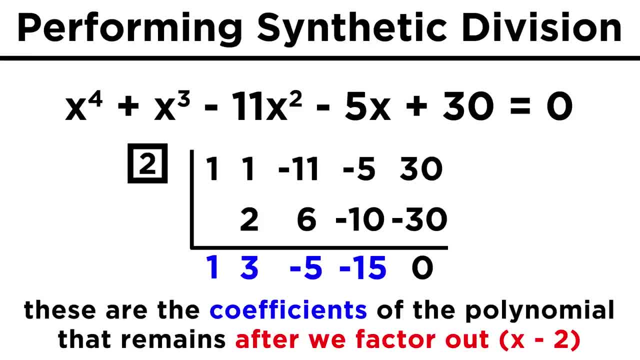 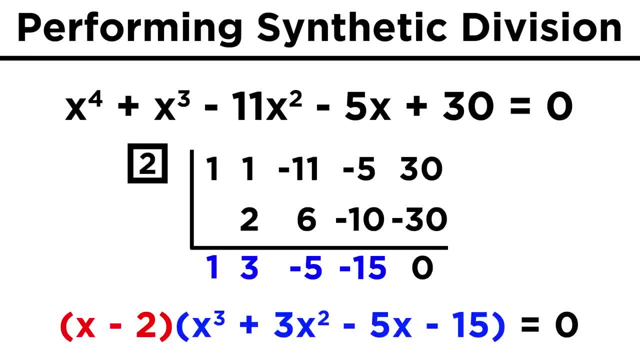 Let's look at them one by one. Let's look at them one by one. If we look at the coefficients of the polynomial that remains after dividing by X minus two, We just have to understand that what is left will be of a degree that is one less than. 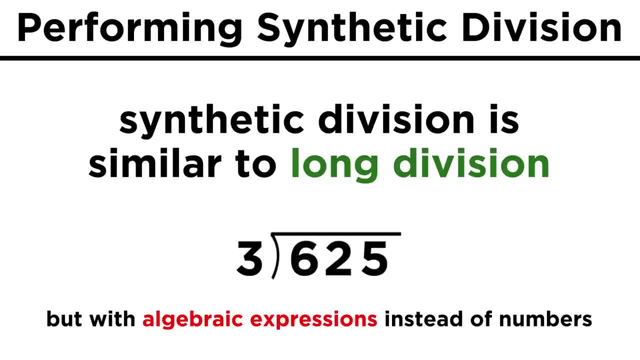 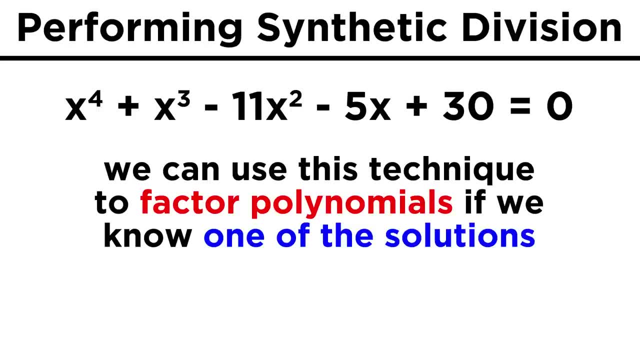 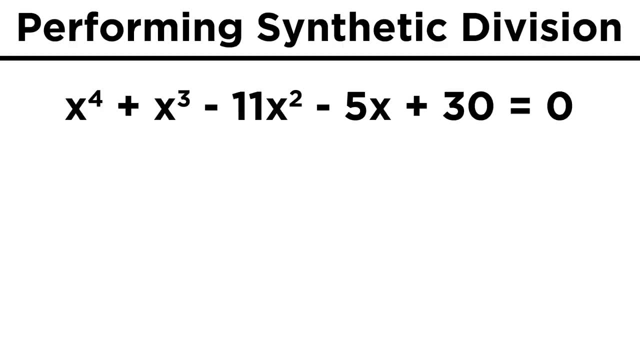 that we are using algebraic expressions instead of numbers. This will come in handy if we have something like a cubic or quadrangle. Let's say we are looking at X to the fourth plus X, cubed minus eleven, X squared minus five, X plus thirty, and we want to see if X equals two is one of the solutions. 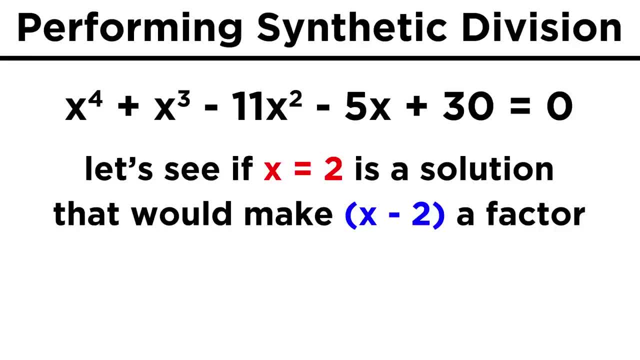 If it is, then X minus two would be a factor, and that could allow us to simplify the expression. The way we will test this is as follows. Let's make two lines at a right angle like this: Let's make two lines at a right angle like this: 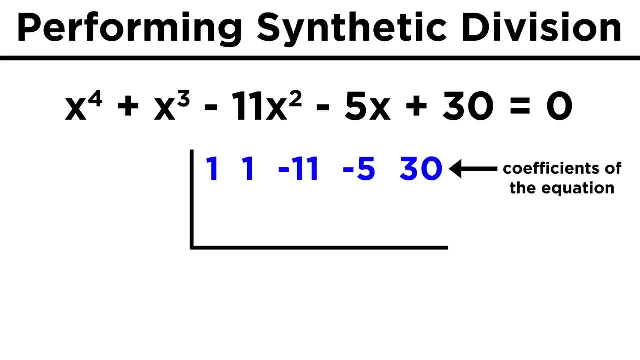 In the top row we will list only the coefficients of our equation. Then we want to test to see if two is one of the solutions. so let's put a two to the left over here. Now we take the first coefficient, in this case a one, and drop it down here. 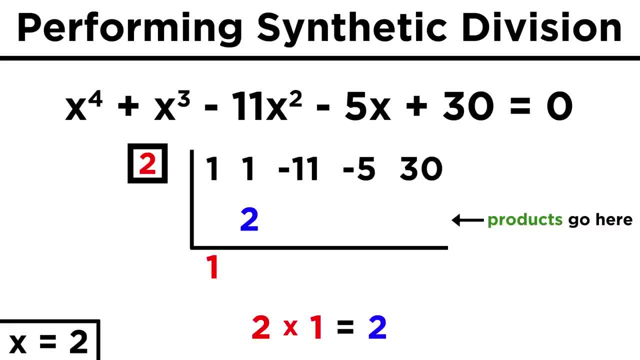 Now we multiply by the two and put that here. Now we can add these together to get three and write that here Again. we multiply by two to get six. Adding to negative eleven. we get negative five. Then we multiply to get negative ten, add to get negative fifteen. multiply to get negative. 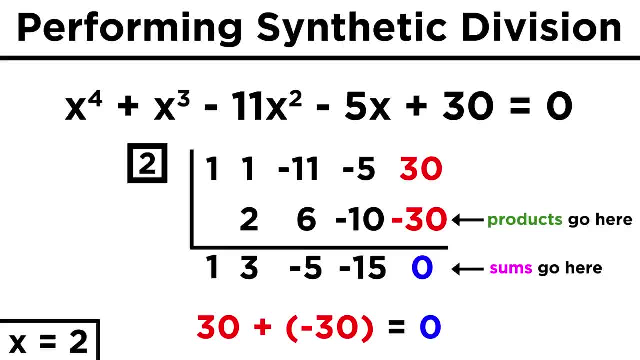 thirty and finally we add to get zero. The fact that this is a zero right here means that there is no remainder from the division, which means that two is a solution, and therefore X minus two is indeed a factor of this polynomial. These resulting numbers here tell us the coefficients. 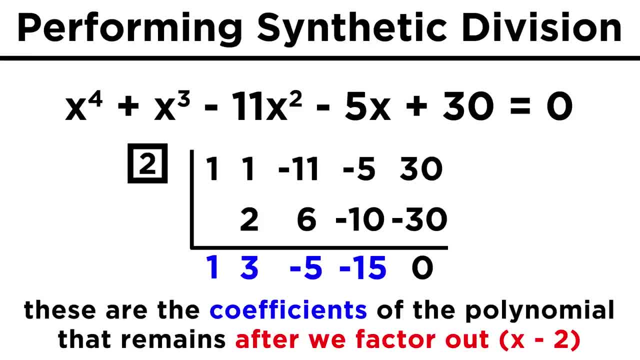 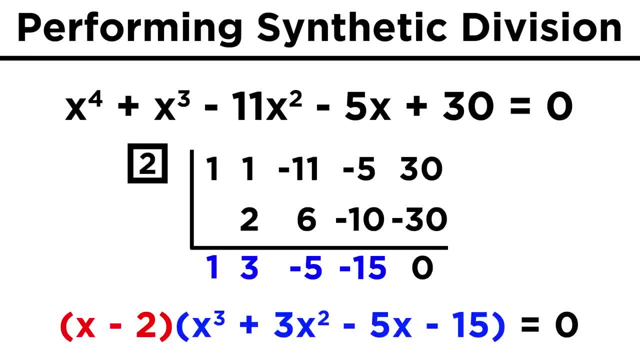 Let's look at them one by one. Let's look at them one by one. If we look at the coefficients of the polynomial that remains after dividing by X minus two, We just have to understand that what is left will be of a degree that is one less than. 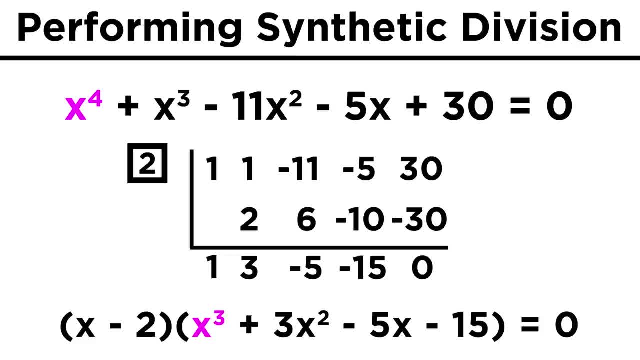 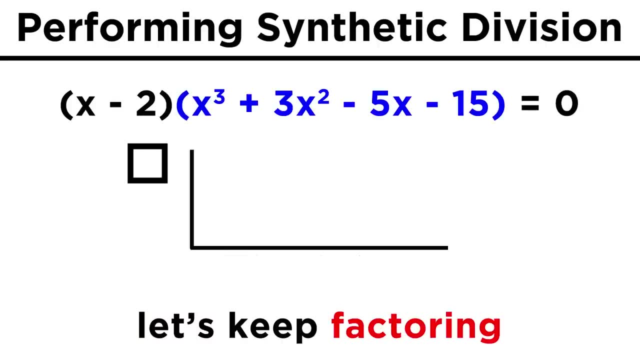 the original polynomial. so since we started with a quartic, the result is a cubic. We can simplify this to: X minus two times X cubed plus three, X squared minus five, X minus fifteen. If we wanted, we could continue factoring. 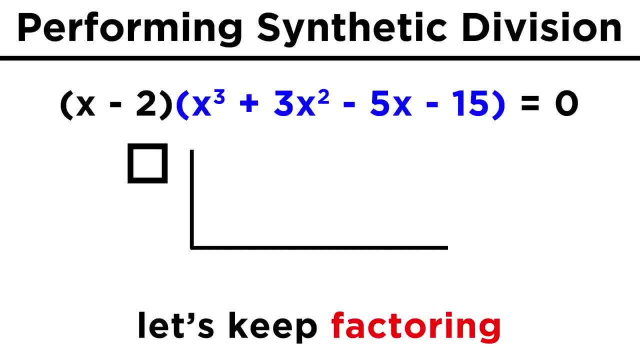 from there until we have nothing but binomials and therefore all the possible solutions. Say we continue with this one and try to see if negative three is a solution. We would perform the same algorithm as before, dropping the one down: multiplying to get. 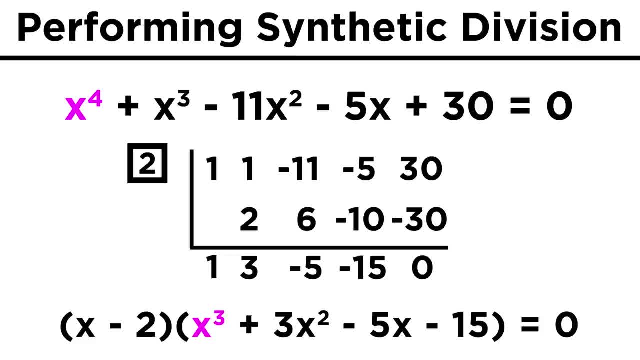 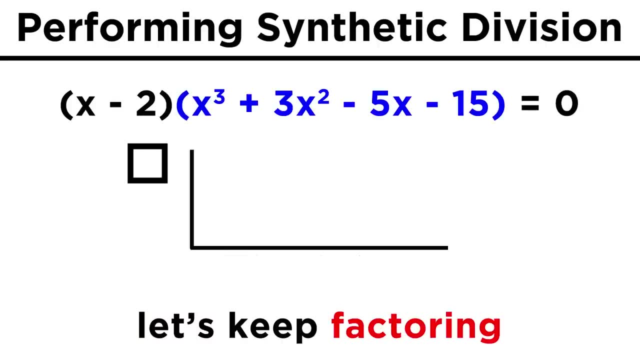 the original polynomial. so since we started with a quartic, the result is a cubic. We can simplify this to: X minus two times X cubed plus three, X squared minus five, X minus fifteen. If we wanted, we could continue factoring. 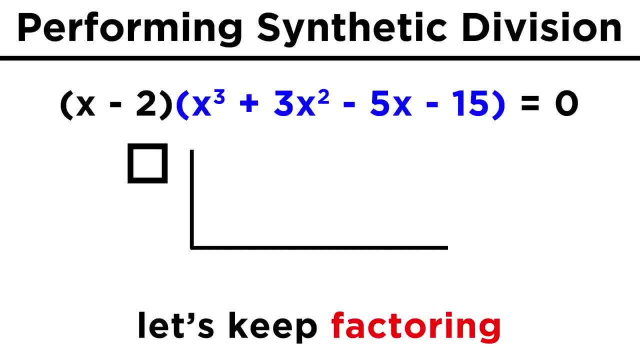 We can continue factoring from there until we have nothing but binomials and therefore all the possible solutions. Say we continue with this one and try to see if negative three is a solution. We would perform the same algorithm as before, dropping the one down: multiplying to get. 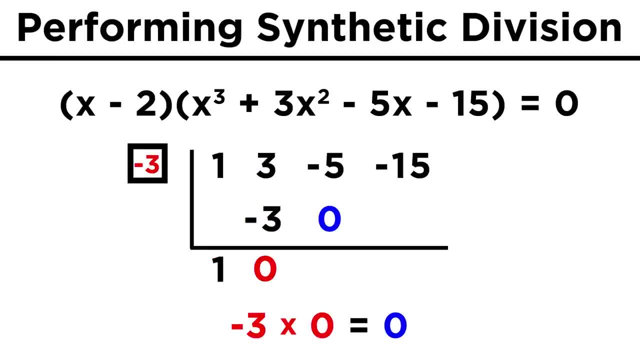 negative three, adding to get zero, multiplying to get zero, adding to get negative five, multiplying to get fifteen and adding to get zero, Once again with a remainder of zero. we see that negative three is indeed a solution and X plus three is therefore a factor. 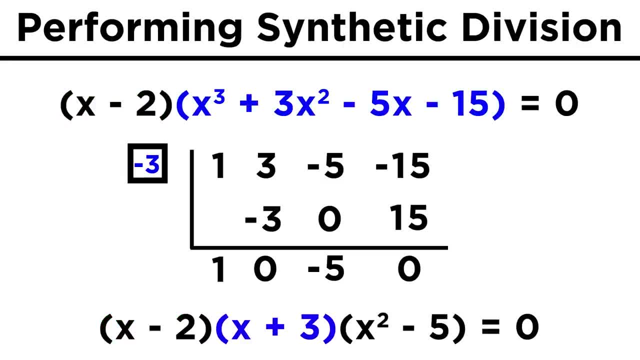 So, leaving the X minus two as it is, we can factor this cubic term further to get X plus three times X squared minus five, which we get from the coefficients we just calculated. That last bit is easy to solve in a separate equation. We just bring five over here, take the square root and we get plus or minus root five. 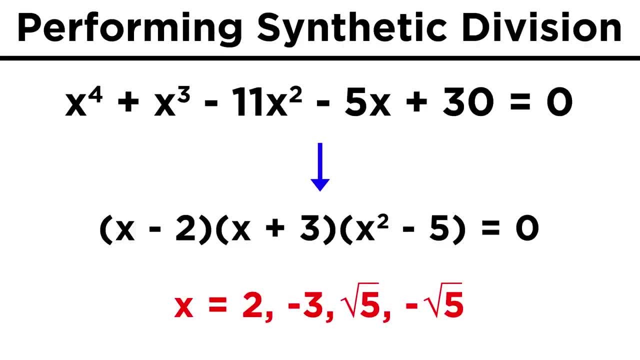 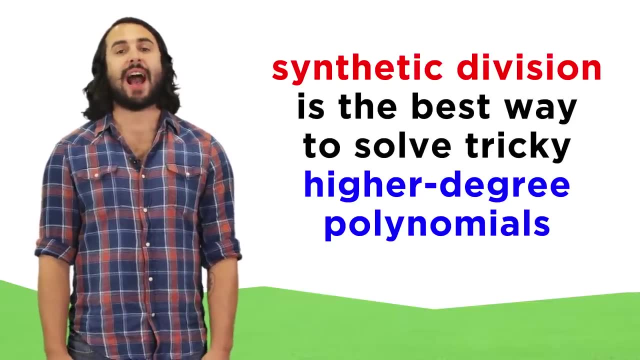 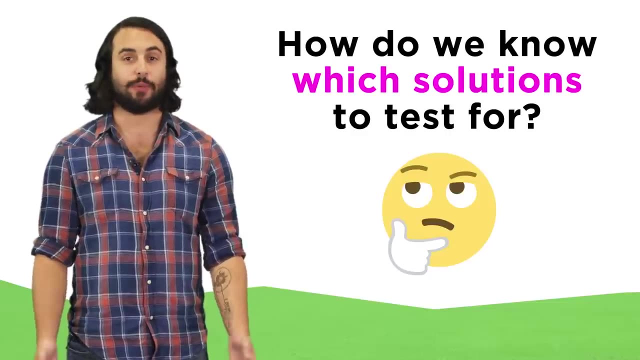 That means we have successfully found all four solutions to this original quartic equation and those are two negative three root five and negative root five. So this is the best way to solve for equations of a degree higher than second degree. You may be wondering how do we decide which possible solutions to test for? 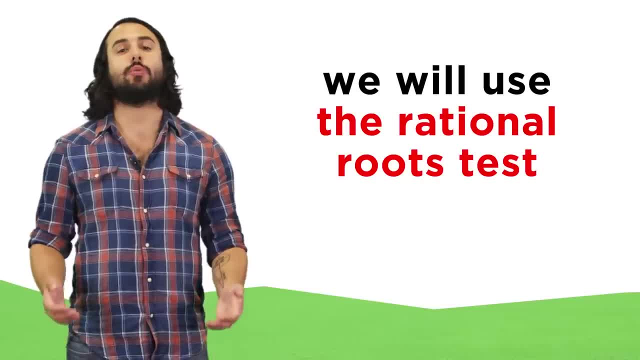 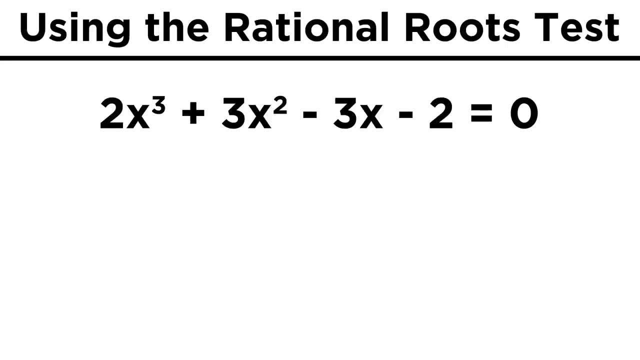 That's a very good question. So let's go over the rational roots test. So let's go over the rational roots test. This is something we can do to get a list of possible solutions. to try To get this list, we just look at the expression like this: one: two X cubed plus three X squared. 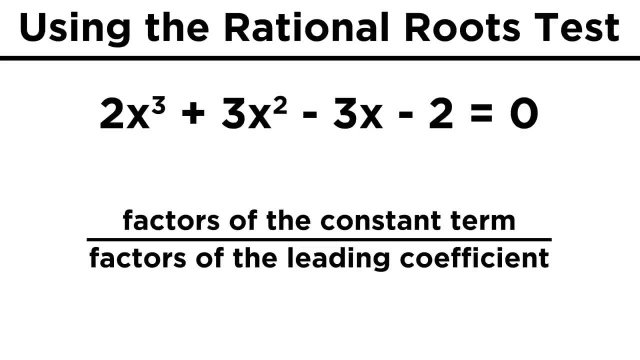 minus three, X minus two, and we make a fraction. On the numerator of this fraction will go all the factors of the constant term, which are one and two. On the denominator go all the factors of the coefficient of the leading term, which are: 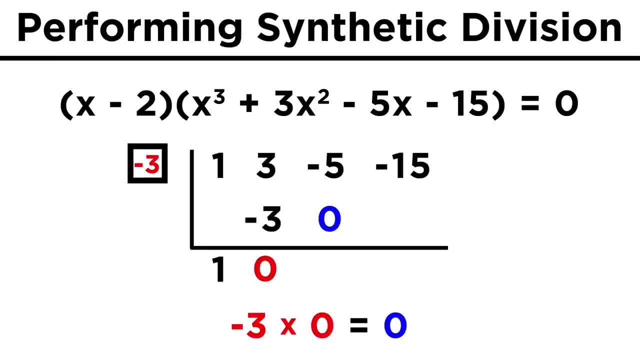 negative three: adding to get zero, multiplying to get zero, adding to get negative five, multiplying to get fifteen and adding to get zero, Once again with a remainder of zero. Well, that's what we want: zero. we see that negative three is indeed a solution and X plus three is therefore. 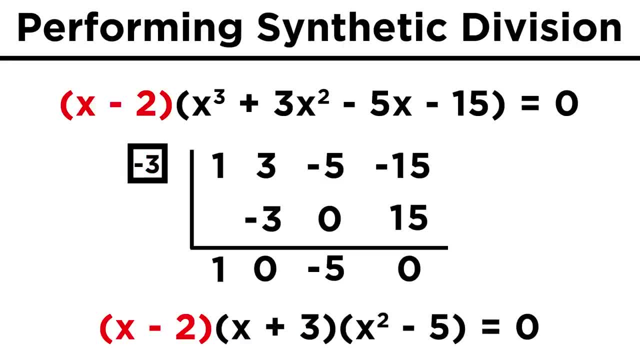 a factor. So, leaving the X minus two as it is, we can factor this cubic term further to get X plus three times X squared minus five, which we get from the coefficients we just calculated. That last bit is easy to solve in a separate equation. we just bring five over here. take: 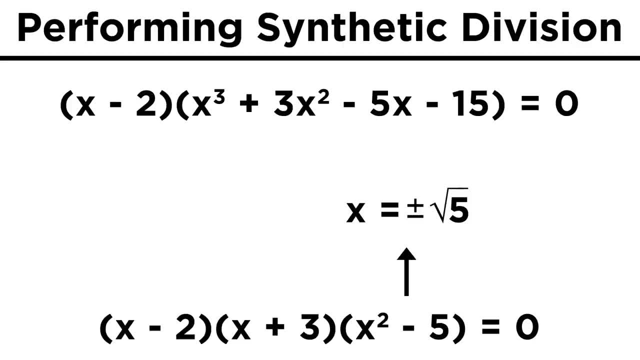 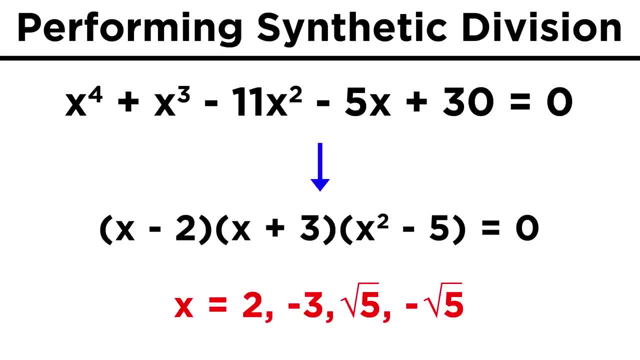 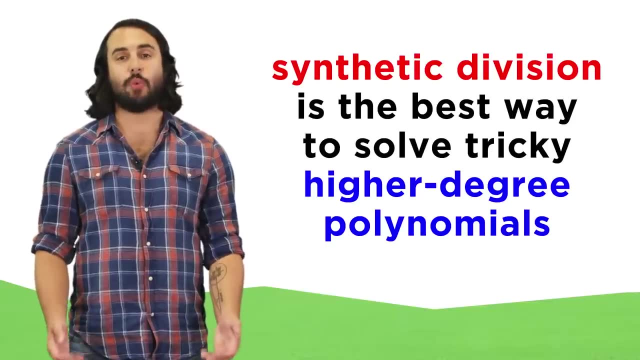 the square root and we get plus or minus root five. That means we have successfully found all four solutions to this original quartic equation and those are two negative three root five and negative root five. So this is the best way to solve for equations of a degree higher than second degree. 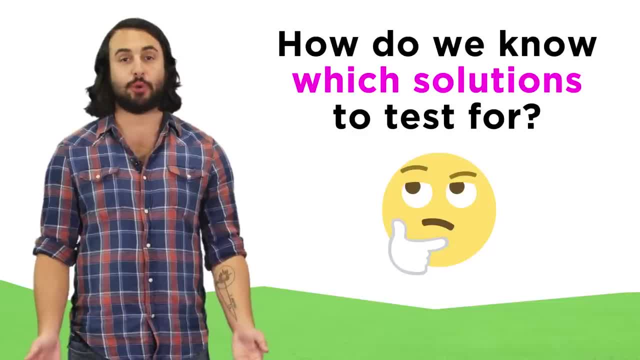 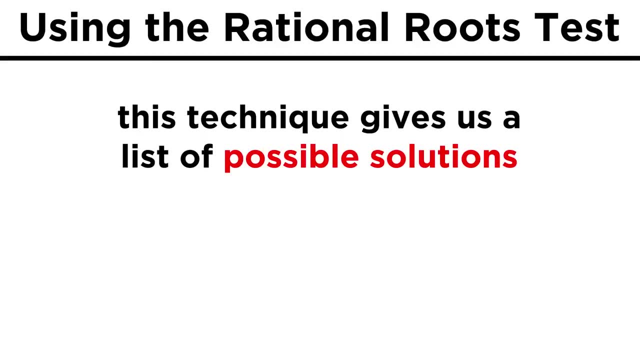 You may be wondering: how do we decide which possible solutions to test? for That's a very good question. So let's go over the rational roots test. This is something we can do to get a list of possible solutions. to try To get this list, we just look at the expression like this one: two X cubed plus three X squared. 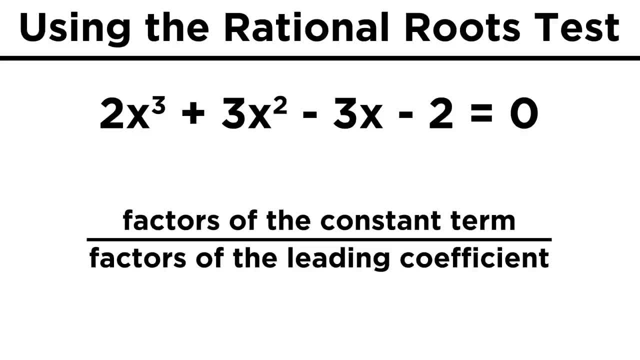 minus three, X minus two, and we make a fraction. On the numerator of this fraction will go all the factors of the constant term, which are one and two. On the denominator go all the factors of the coefficient. On the denominator go all the factors of the coefficient of the leading term, which are: 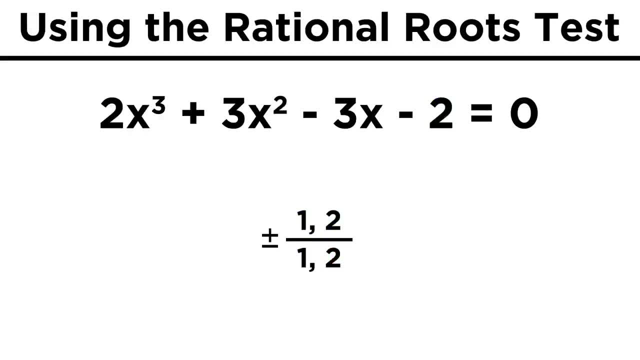 again one and two. We also put a plus or minus to the left of this fraction To get all the likely zeros to test. we just make all the possible fractions. So we could try: plus or minus one, plus or minus one half and plus or minus two. 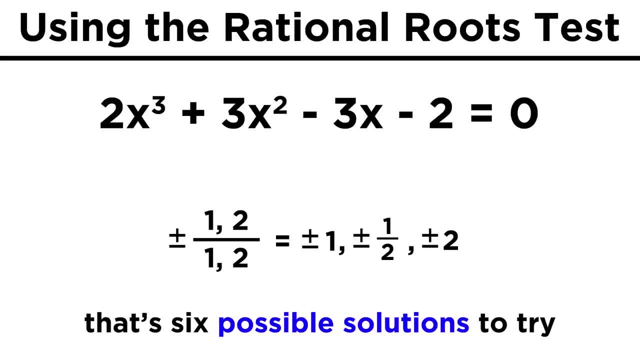 That is still six possibilities to try, but at least it gives us a short list of good options. Remember, these are not all solutions, Just a list of possible solutions. Sometimes none of these will end up being solutions. It's just a helpful trick that will usually shorten our search. 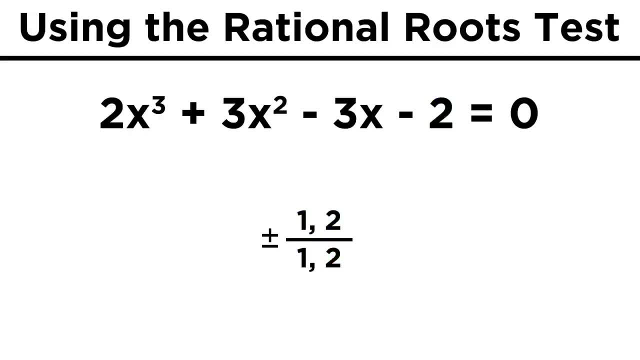 again one and two. We also put a plus or minus to the left of this fraction To get all the likely zeros to test. we just make all the possible fractions. So we could try: plus or minus one, plus or minus one half and plus or minus two. 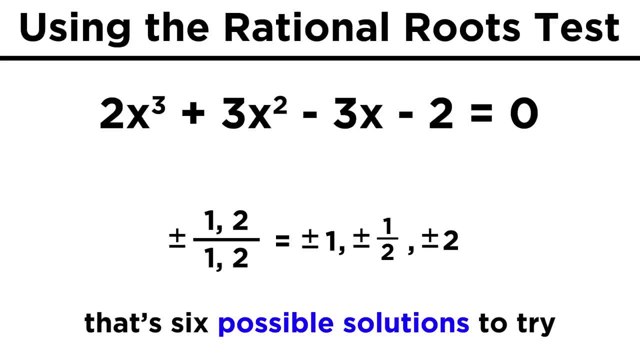 That is still six possibilities to try, but at least it gives us a short list of good options. Remember, these are not all solutions, just a list of possible solutions. Sometimes none of them are possible. Sometimes none of them are possible. 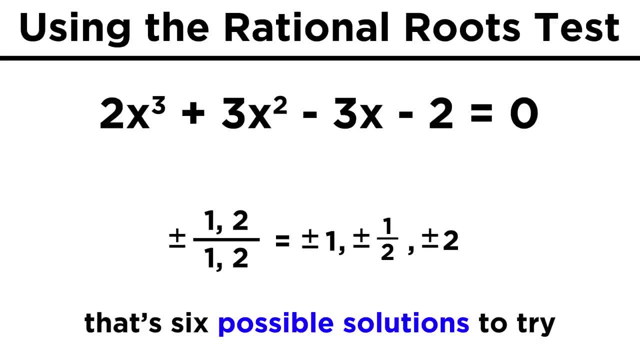 Sometimes none of these will end up being solutions. It's just a helpful trick that will usually shorten our search. Let's try and see if X equals one is a solution. We do our synthetic division by setting things up as we learned before with the coefficients. 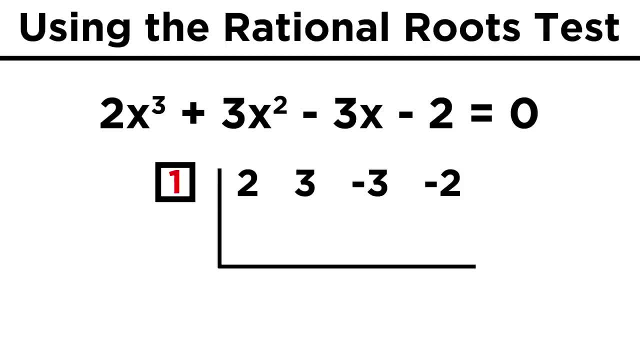 two, three, negative three and negative two. We place the one here, drop the first two down and get to multiplying and adding. One times two is two. Three plus two is five. One times five is five. Negative. three plus five is two. 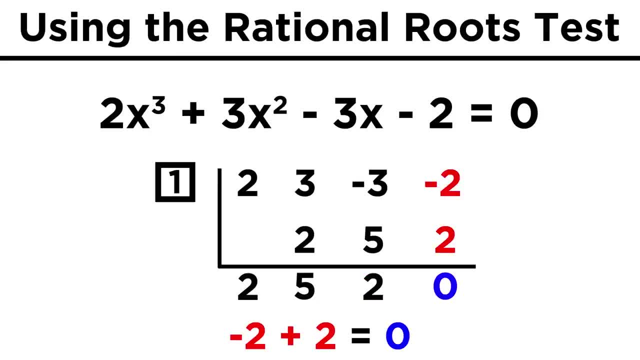 One times two is two And negative two plus two is zero. That means that one is indeed a solution. Remember, if this last digit was anything other than zero, then the number you are testing is not a solution. You can cross it out and try something else from the list. 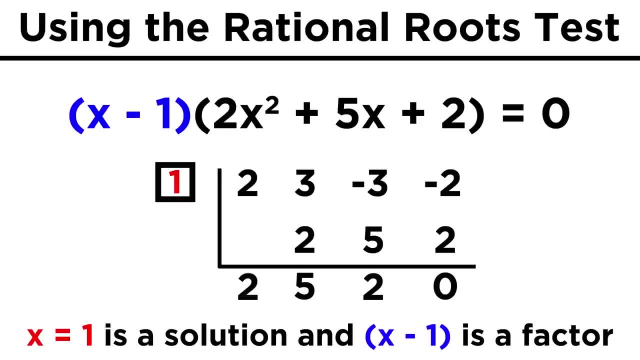 But this one did work, so we can split up this cubic function into X minus one, since one was a solution. X minus one is zero, A quadratic function given by the coefficients here, which will be two X squared plus five X plus two. 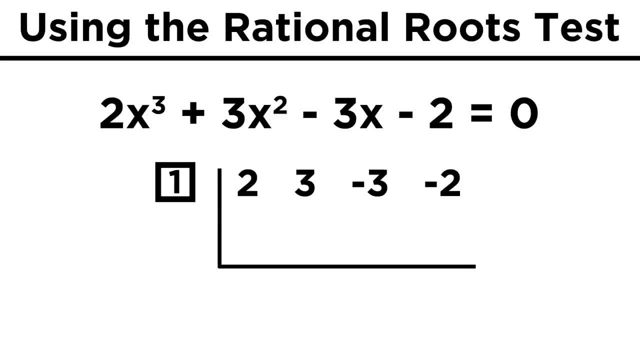 Let's try and see. if X equals one is a solution. We do our synthetic division by setting things up as we learned before with the coefficients two, three, negative three and negative two. We place the one here, drop the first two down and get to multiplying and adding. 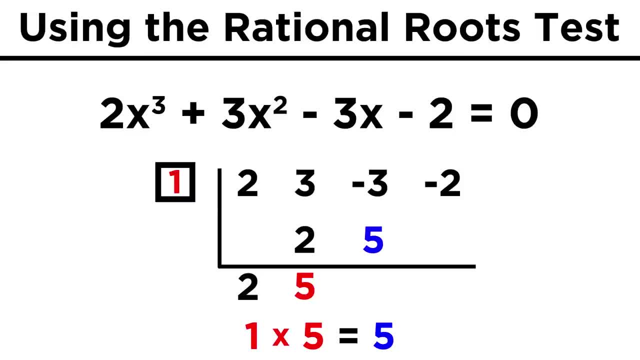 One times two is two. Three plus two is five. One times five is five. Negative three plus five is two, One times two is two And negative two plus two is zero. That means that one is indeed a solution. Remember, if this last digit was anything other than zero, then the number you are testing. 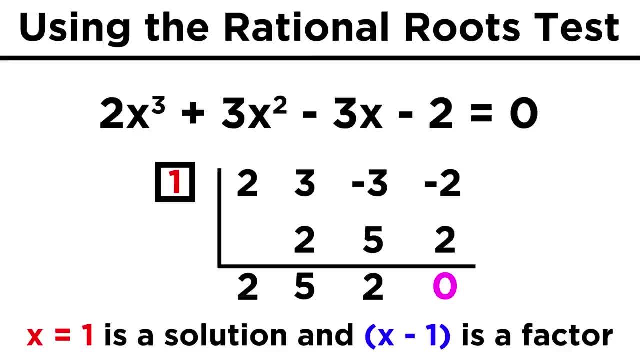 is not a solution. You can cross it out and try something else from the list, But this one did work. So we can split up this cubic function into X minus one and negative. two plus two is zero, And then a quadratic function given by the coefficients here, which will be two X squared. 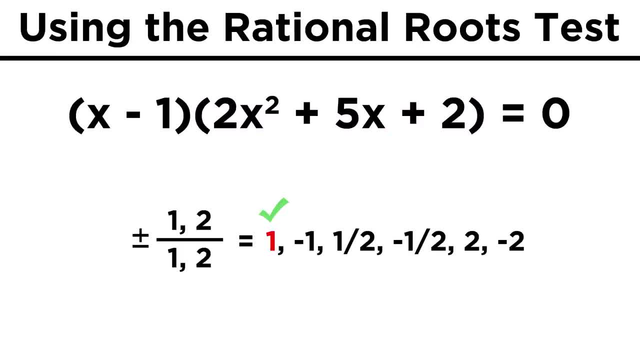 plus five, X plus two. From there we could go back to our list of zeros and try another. Perhaps negative two will work, So we can keep the same workspace. put a negative two here, drop the two down and off we go. 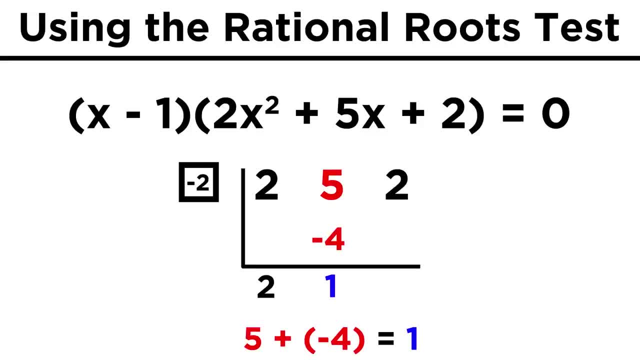 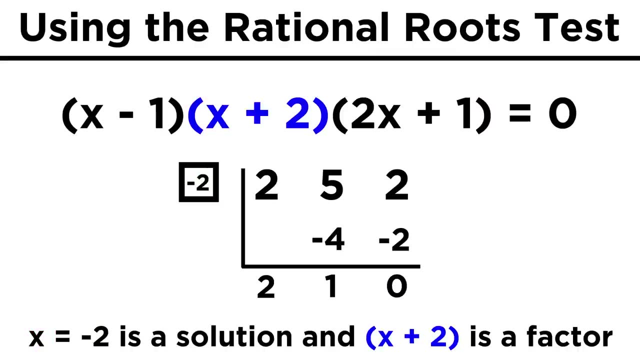 Negative two times two is negative four. Five plus negative four is one. Negative two times one is negative two. Two plus negative two is zero. Once again, the zero means that this is a solution. so we can break this quadratic up into X plus two, since negative two is a solution and the resulting binomial from synthetic. 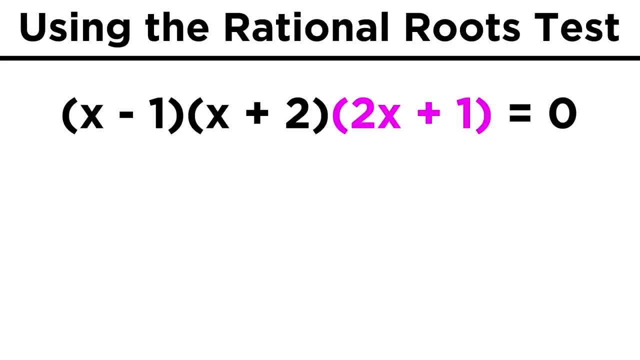 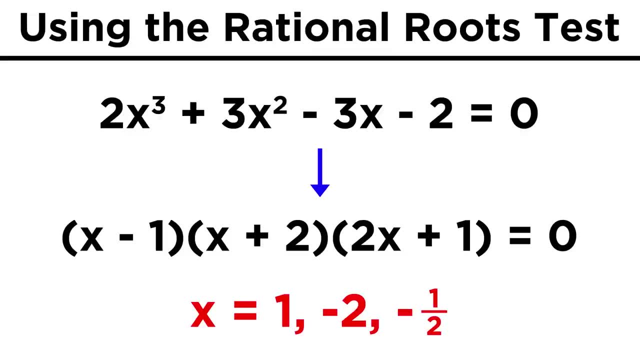 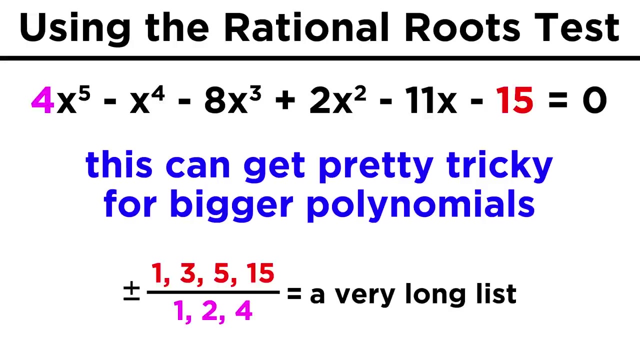 division two X plus one. Looking at this last binomial, it is clear that if we solve this term by itself, we get negative one half, and so the three zeros, or solutions of this quadratic equation, are negative one half. You can imagine how this can get much trickier for quartics or quintics, especially if the 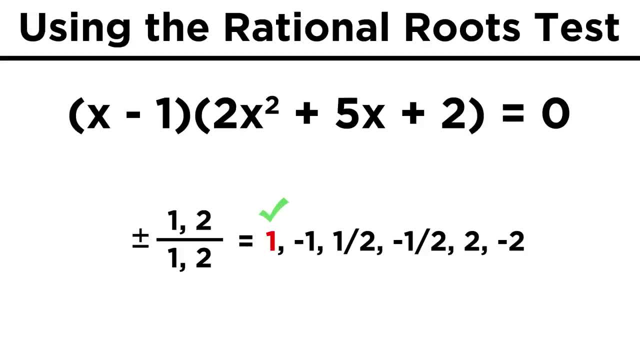 From there we could go back to our list of zeros and try another. Perhaps negative two will work, So we can keep the same workspace. put a negative two here, drop the two down and off we go. Negative two times two is negative four. 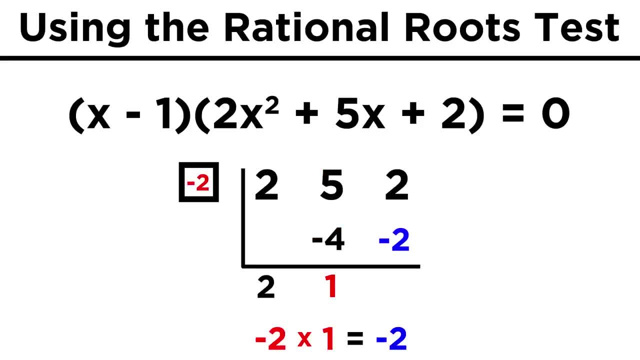 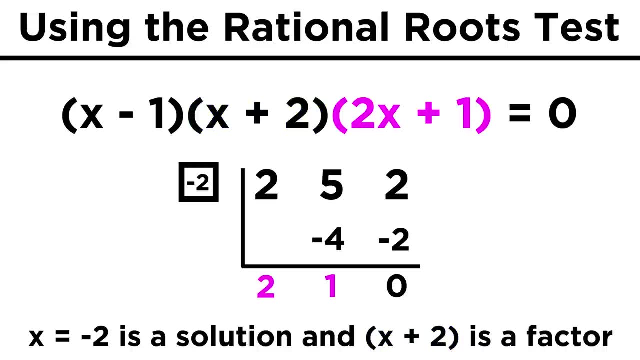 Five plus negative four is one. Negative two times one is negative two. Two plus negative four is one. X plus negative two is zero. Once again, the zero means that this is a solution. so we can break this quadratic up into X plus two, since negative two is a solution and the resulting binomial from synthetic.